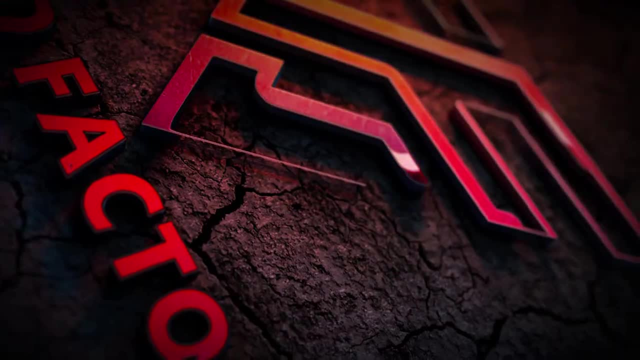 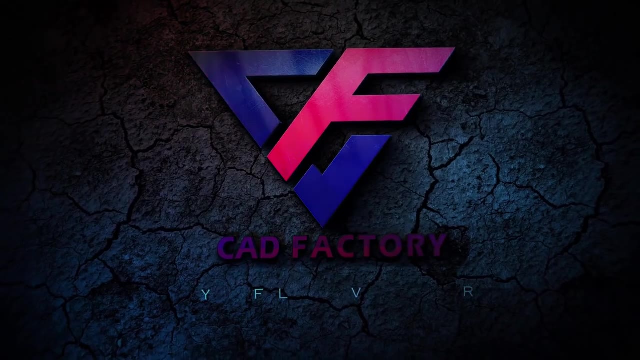 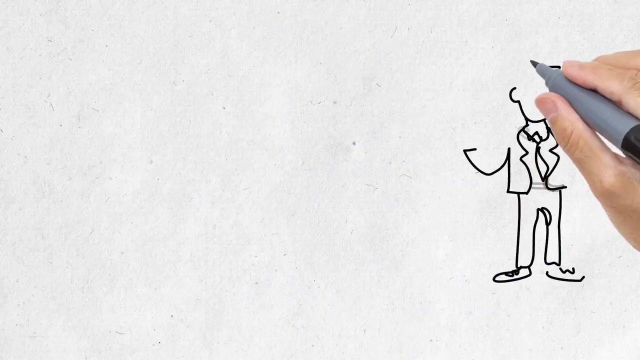 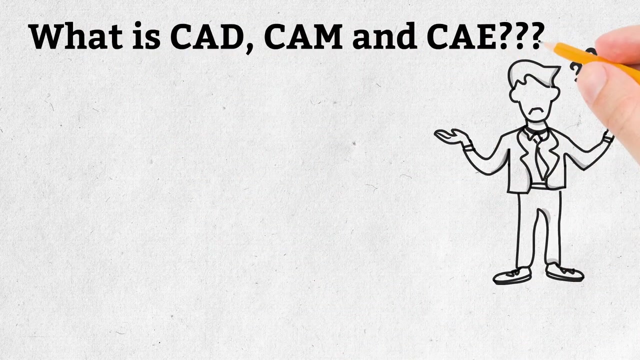 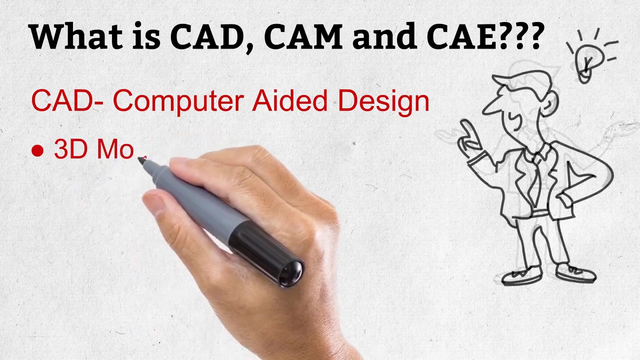 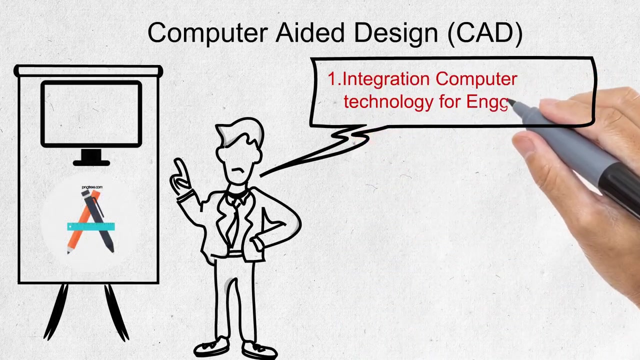 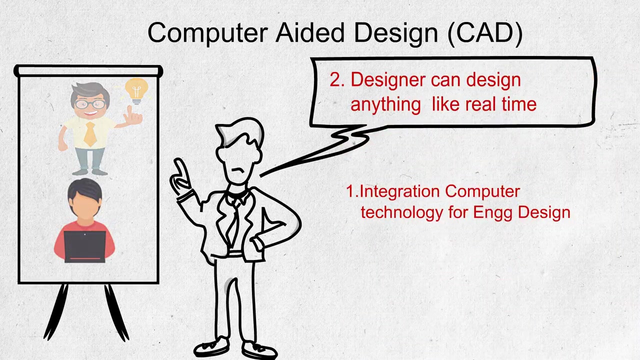 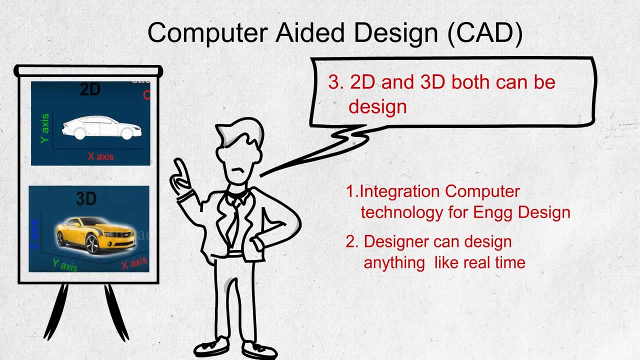 What is CAD, CAM and CAE CAD, Computer Aided Design? It deals with the 3D modeling, CAD design integrated with computer technology and engineering design CAD, which, through design, can design anything like real-time with accuracy. In CAD softwares, both 2D and 3D dimension can be designed. 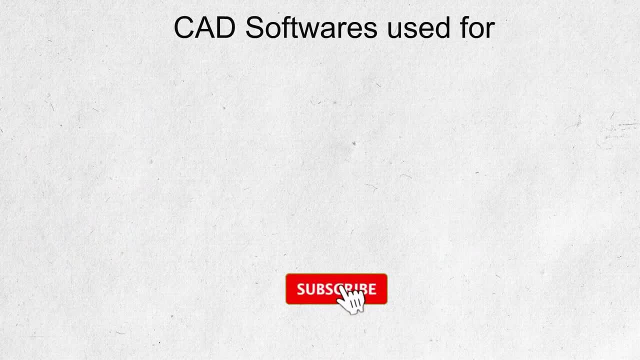 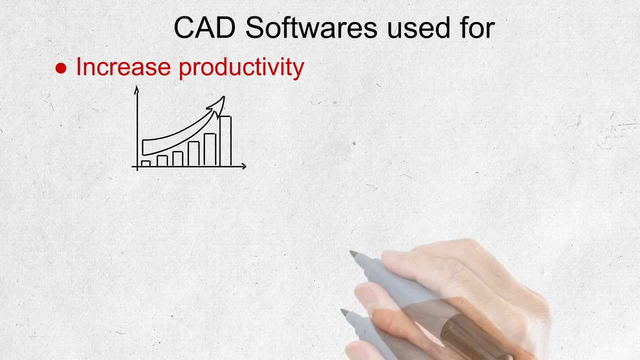 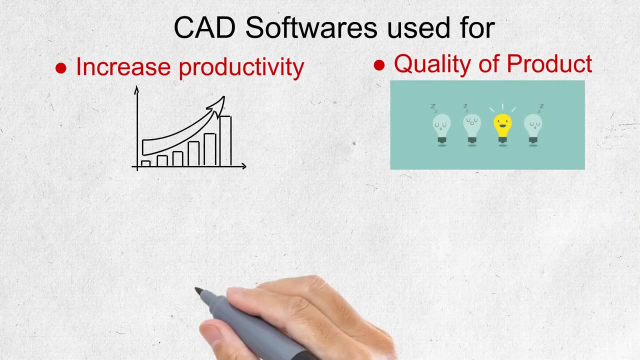 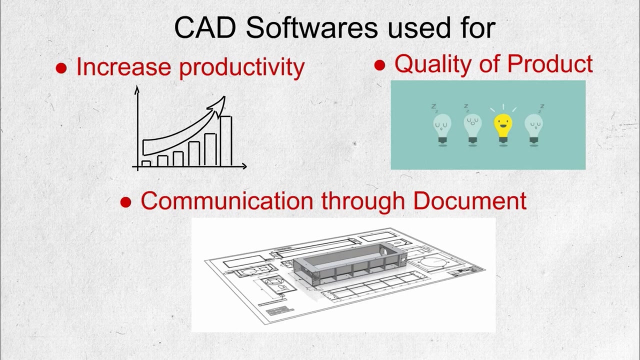 Usage and advantages of CAD softwares. CAD software allows designers to work faster and smarter. CAD softwares allows design teams to control the quality of the final engineered product. The measurements, angles and dimensions of a product are all conveniently recorded and saved for future use. 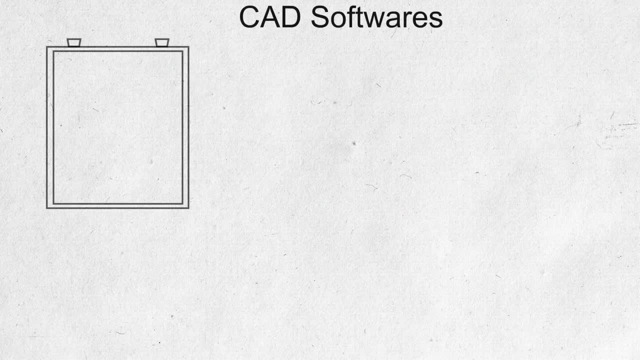 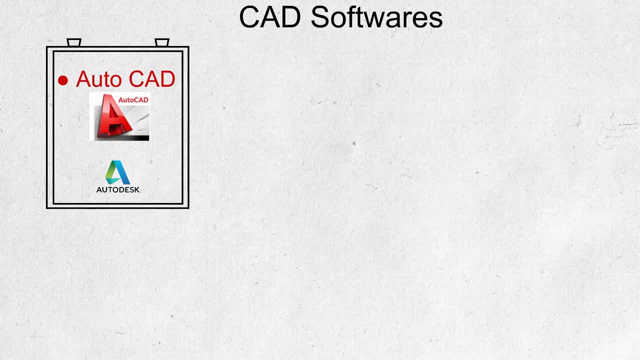 Basic software for both 2D and 3D. Basic software for both 2D and 3D: Click the link in the description. Auto-CAD developed by Autodesk. Classic software developed by Solidworks: 틴 Solidworks. 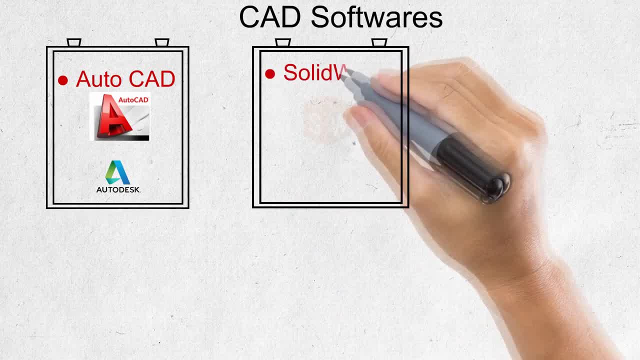 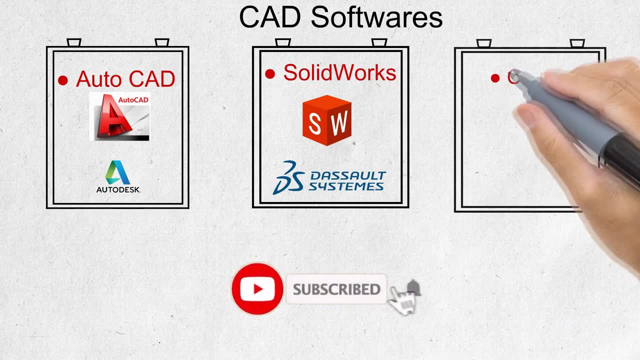 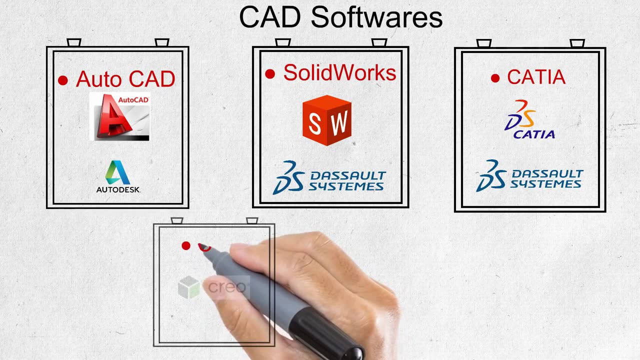 Study the solutions. Tucson Out our platform, search sarasota out or suizec père. We are a vibrant and unique web service. Thank you for listening. This is the Beef esede. Keep up withS�리 вер Loveave. 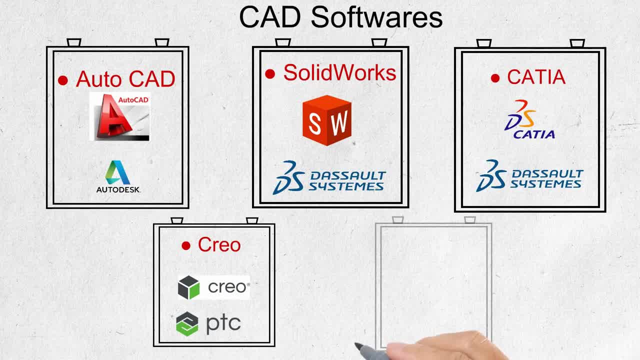 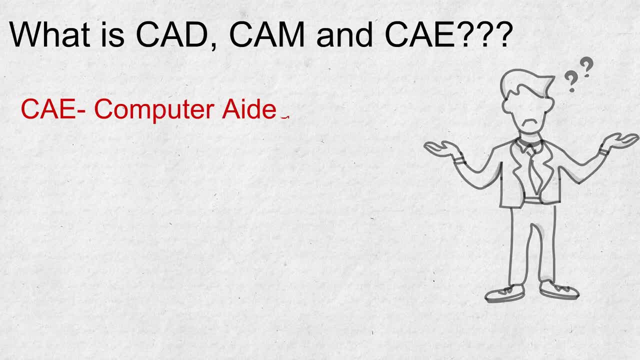 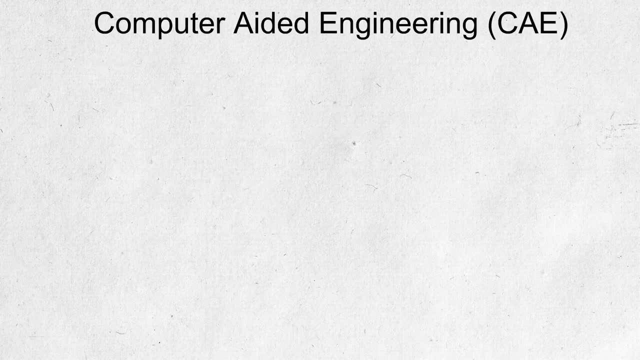 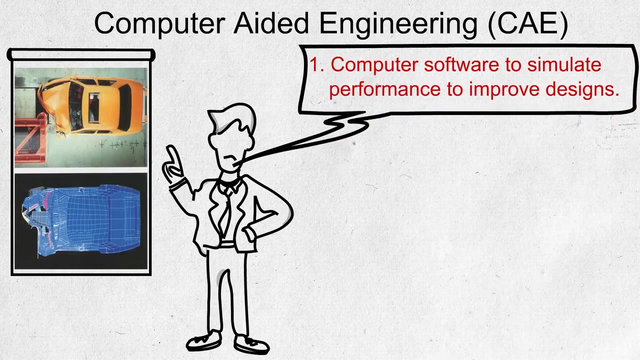 Stretch היא Pro E software. Final one is NX CAD. It's developed by Siemens. next one, CAE Computer-aided engineering. It's deals with analyze the 3d model. No one likes me CAE's computer software to simulate the performance in order to improve product designs. 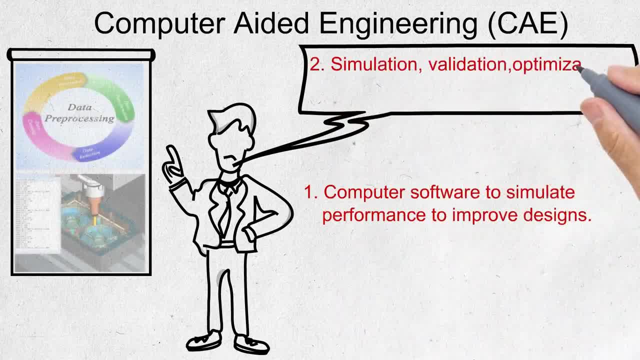 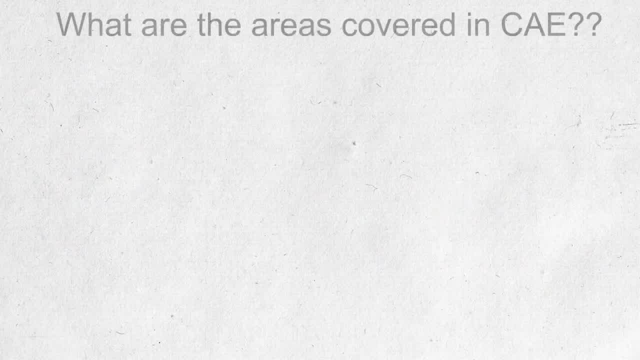 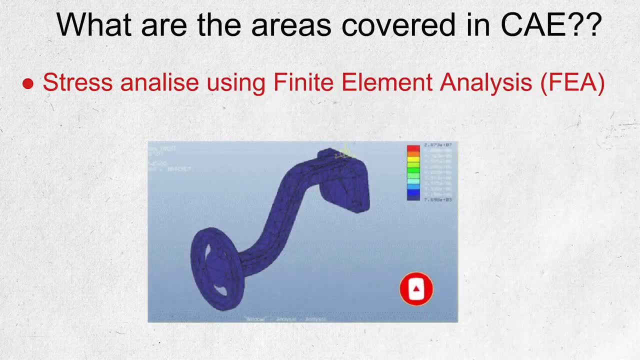 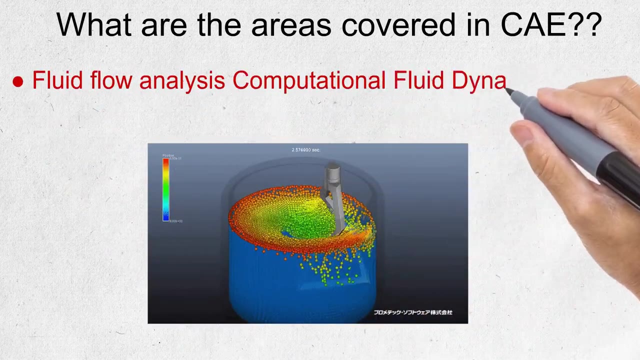 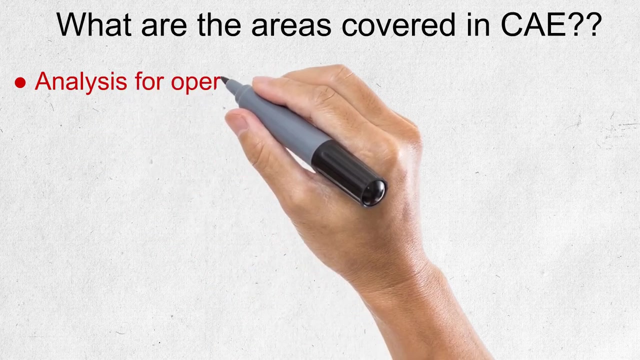 CAE also consider simulation, validation and optimization of products and manufacturing tools. What are the areas covered in CAE? stress analysis on components and assemblies using finite element analysis, FVA. thermal with fluid flow analysis, computational fluid dynamics. CFD Analysis. tools for Process simulation for operations such as: 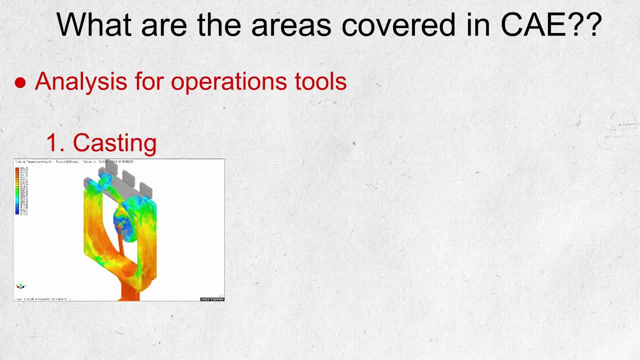 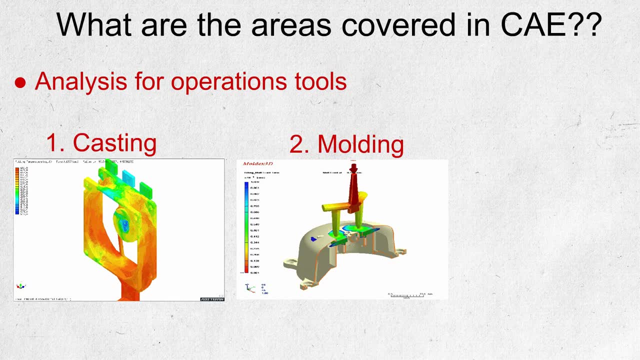 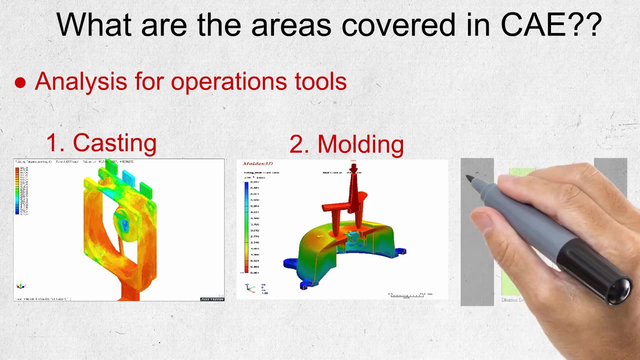 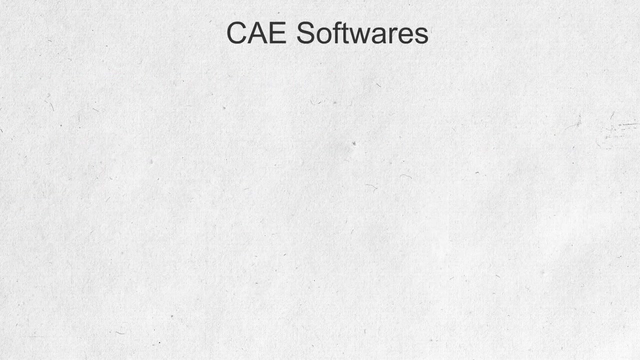 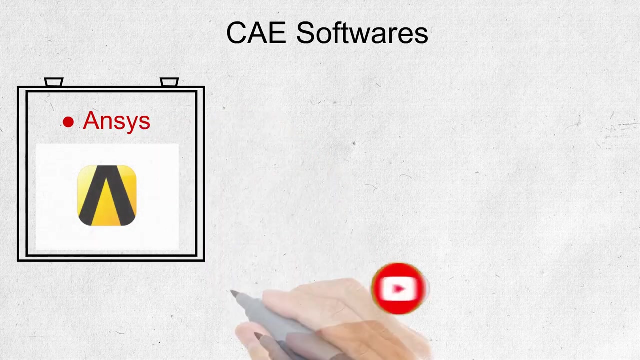 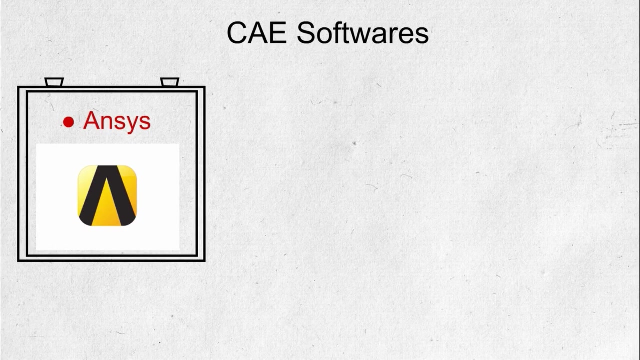 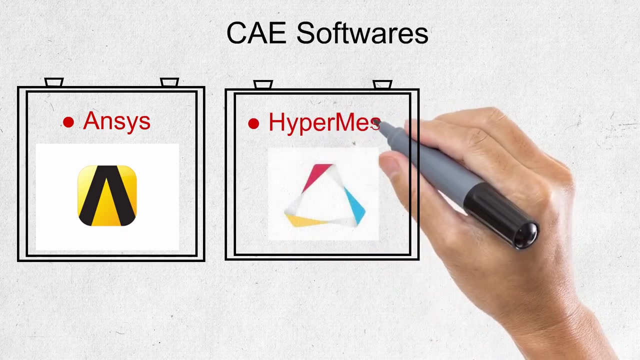 CAE: Sting, Molding And die press. What are the software Available in CAE? First one is ansys: it's analyzing strength, toughness, elasticity, temperature distribution, electromagnetism, fluid flow and other attributes. next one is Hyper mesh: It's capable of producing meshes that are high quality, made with no complexity. 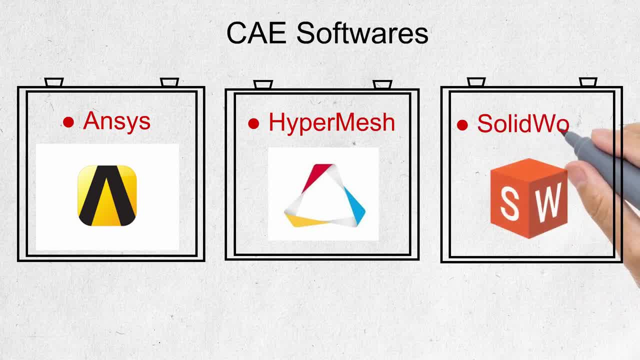 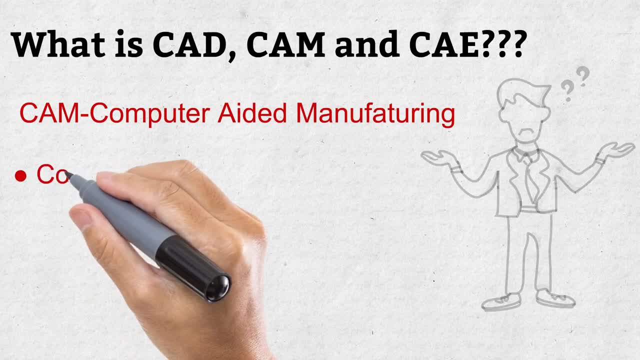 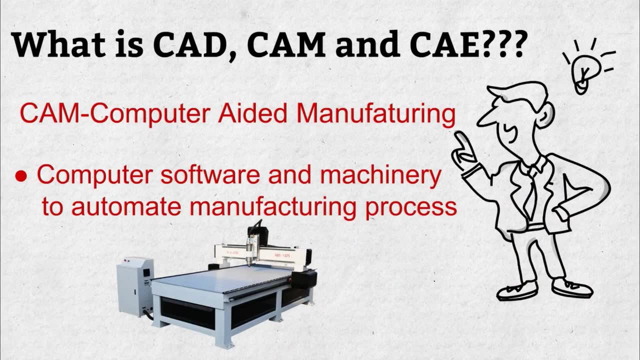 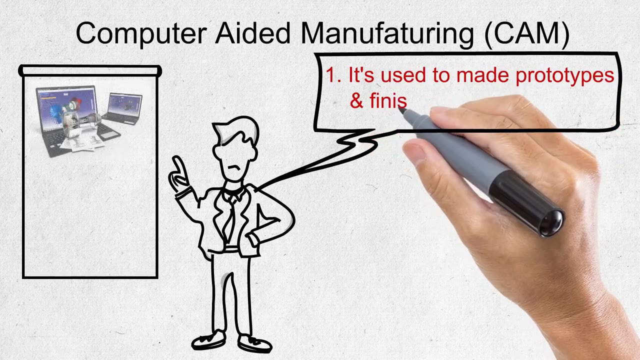 next one is Solid works developed by Dassault System. Finally, CAM- Computer Aided Manufacturing. CAM is an application technology that uses computer software and machinery to automate manufacturing processes. CAM software is used to design and manufacture prototypes, finished products and production runs. 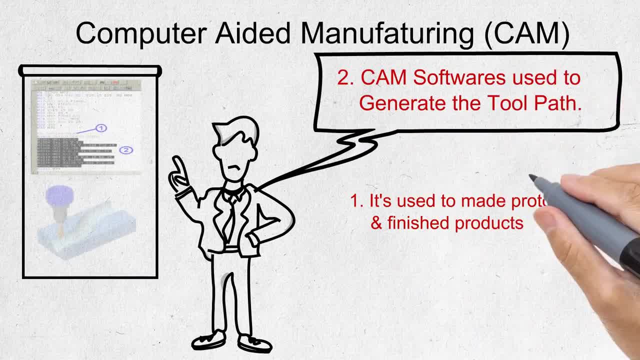 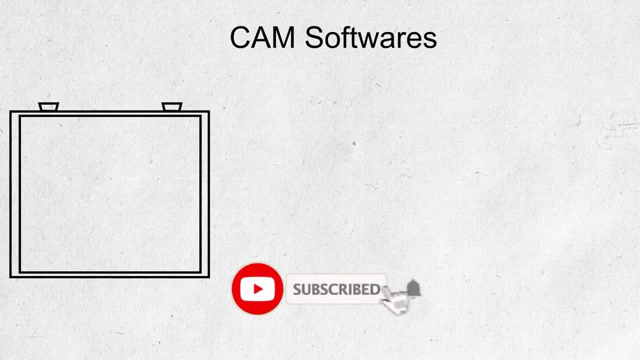 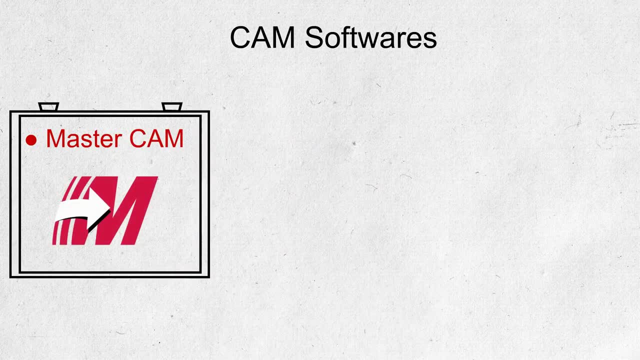 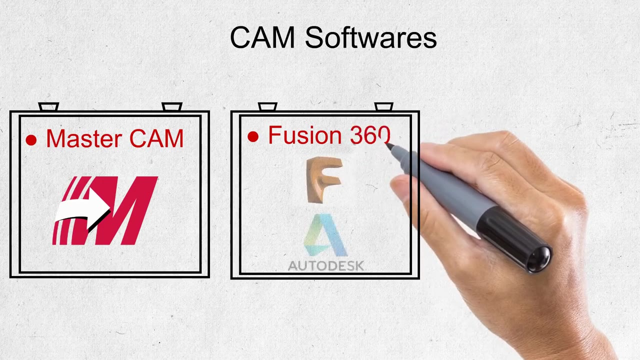 Software that tells a machine how to make a product by generating toolpaths. Now see what are the few softwares available in CAM. First one is Master CAM. it allows for quicker modifications to making the part on the CNC machine. Next one is Fusion 360, it's developed by Autodesk. it's working simultaneously 5 axis for manufacturing process. 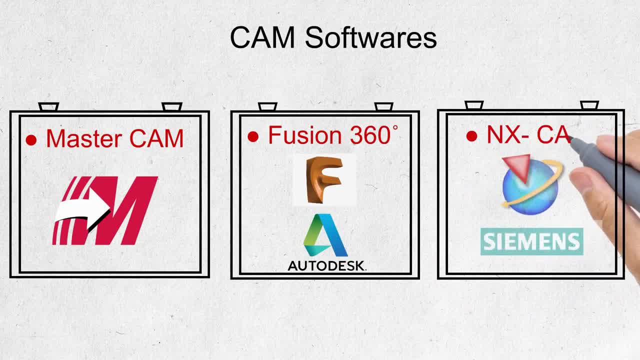 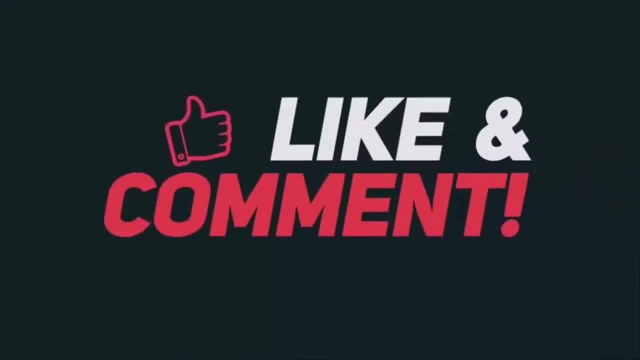 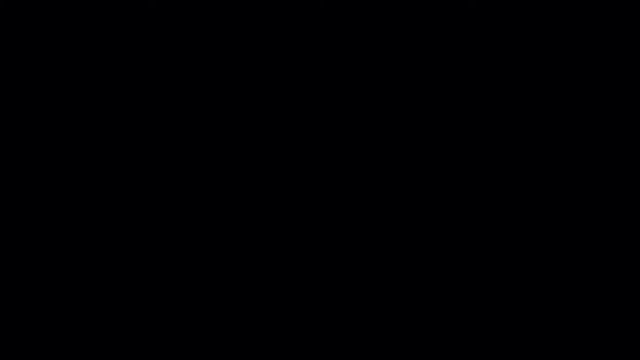 And final one is NX CAM. it's developed by Siemens. Thanks for watching.